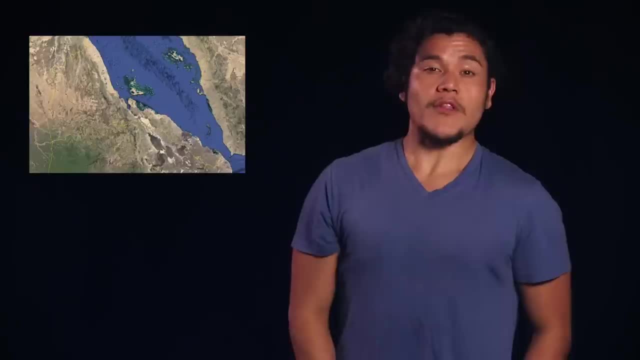 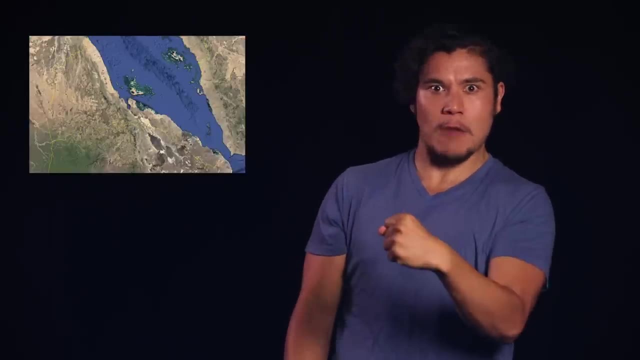 I mean the South Red Sea region is kind of classified as one of the hottest areas on the planet. Nonetheless, they take their coastline seriously. When you own land along one of the busiest trading routes on the planet, you tackle that bad boy and tariff it like a boss. 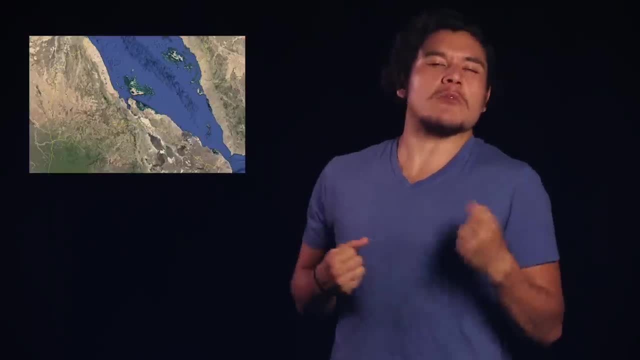 I mean, unless your constituents kind of start hating you and then they put up an embargo but hey, they'll come crawling back. They even set up camp and even have an exclave on the southernmost border with Djibouti, on the Dumaira Peninsula. 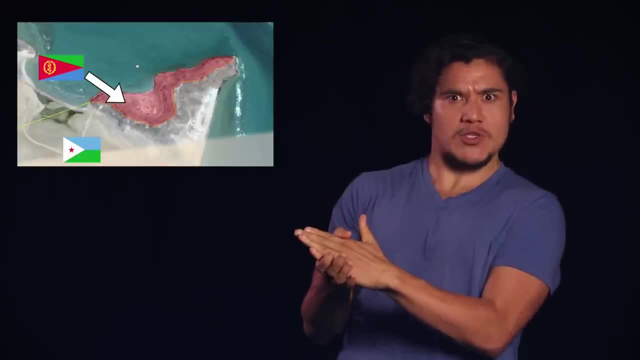 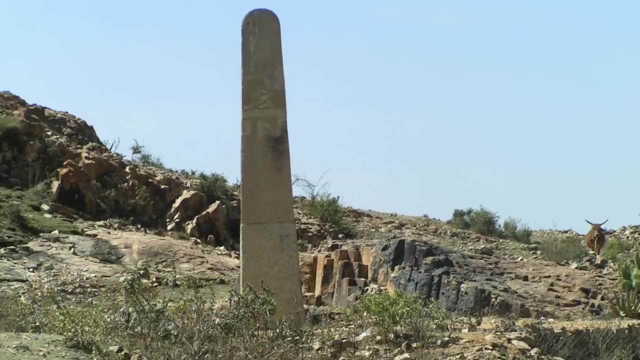 because they were like. We want to get as close as we can to the Bab al-Mandab Strait, Home to quite a few archaeological sites like the ones in Kohaito, Matara and Sanafe, with the Aksumite ruins, many of which are yet to be explored. As well as a plethora of centuries-old churches, monasteries, mosques and mausoleums hidden along the cliffs on the outskirts of towns. The point is, with whatever land that they do have, they work to the best of their ability to feed their ever-growing population. 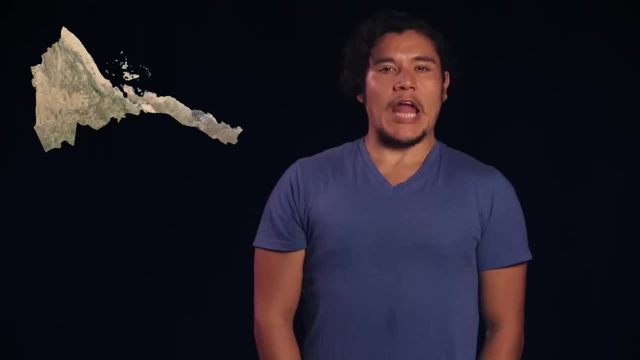 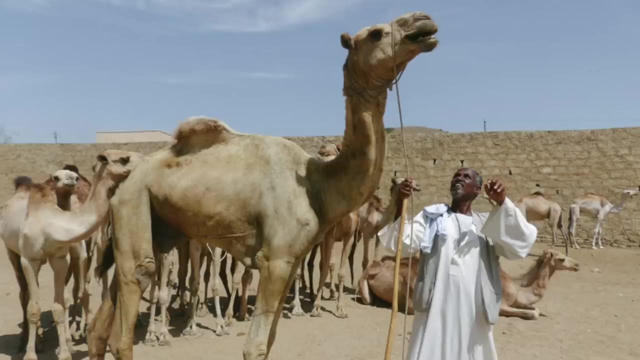 Let's explain Now. yes, as mentioned before, many of the places in Eritrea's coast are generally hot and dry, which, to no surprise, is why the camel is actually the national animal. But that's only one part of the country. Surprisingly, they have quite a contrasting land makeup. 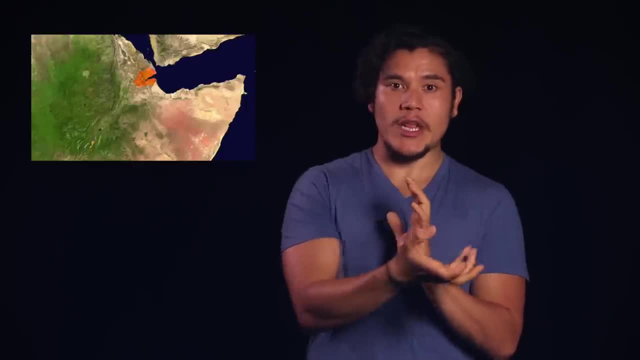 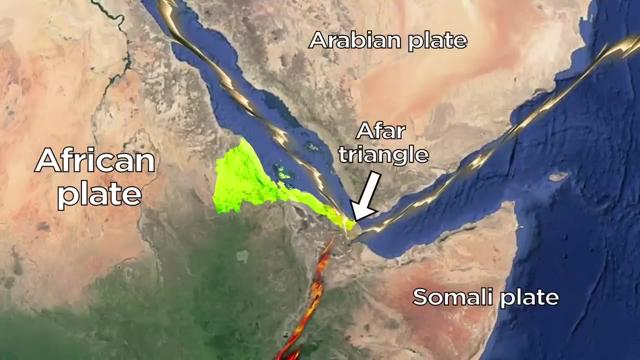 Just like we mentioned in the Djibouti episode, the general area that Eritrea is located in is a hot mess when it comes to three tectonic plates: The Somali, African and Arabian. All three of these converge into an area known as the 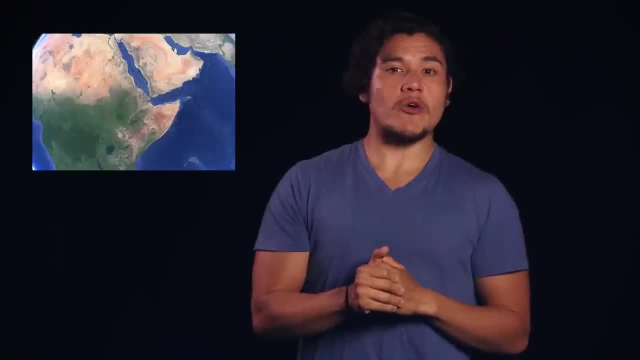 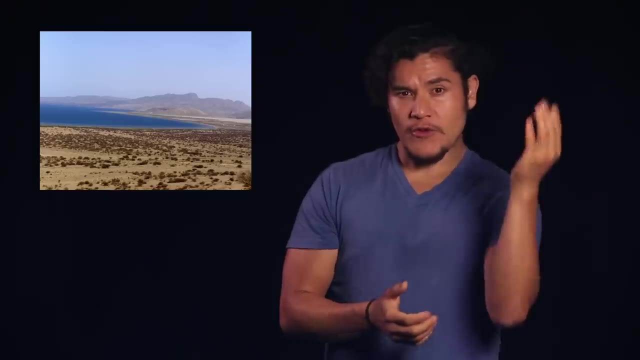 Far Triangle. Basically, the land is tearing itself apart. Eritrea is located right at the fork of the East African Rift, including the Danakil Depression shared with Ethiopia, being labeled as the hottest place on Earth. Therefore, the rift creates coastal highlands. 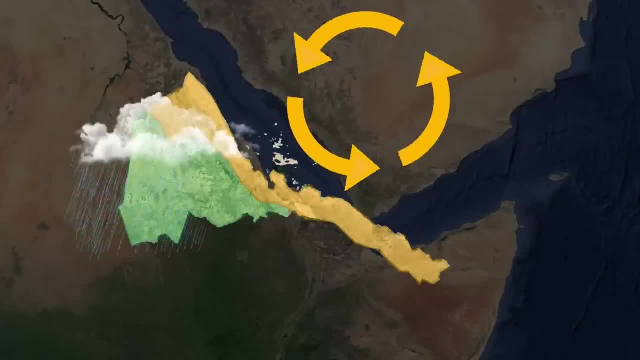 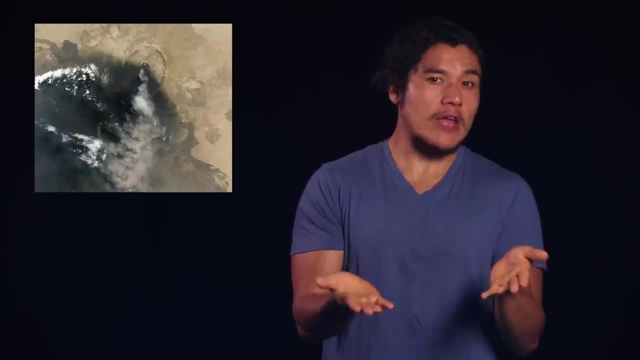 The result looks like a backwards rain shadow effect, in which the coasts are dry and hot and the inland areas are fertile and green. This is also why the majority of the population lives inland. In addition, this gives Eritrea a few volcanoes, most of which are Holocene and extinct. 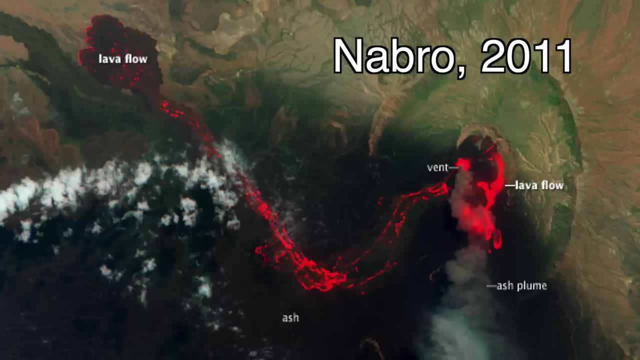 but then again Nabra was thought to be extinct until it kind of went buck wild in 2011.. Inland you can find a range of landmines. You can find landscapes from subtropical rainforests like the ones at Filfil. 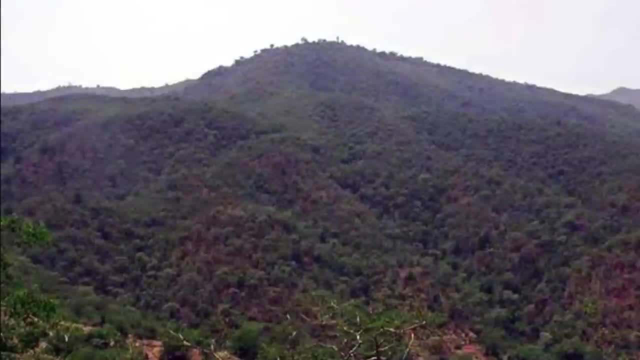 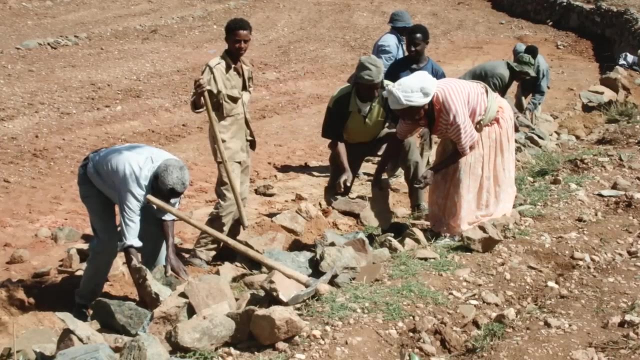 or you can find green, precipitous cliffs and canyons in the Southern Highlands. Despite the lush interior, there still is an issue with desertification and drought. The entire population is required by law, starting at age 15,, to take a month off and terrace hillsides with rocks to prevent erosion and hold in moisture. 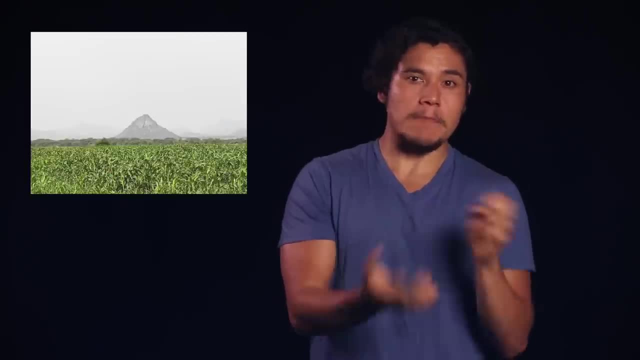 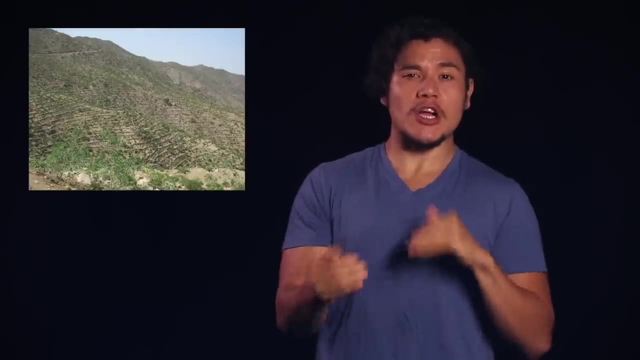 80% of the people live off of agriculture in which crops like barley beans, lentils, sorghum and the interestingly small grain teff is grown. Animals thrive in many parts of the country, especially in the lush interior regions. 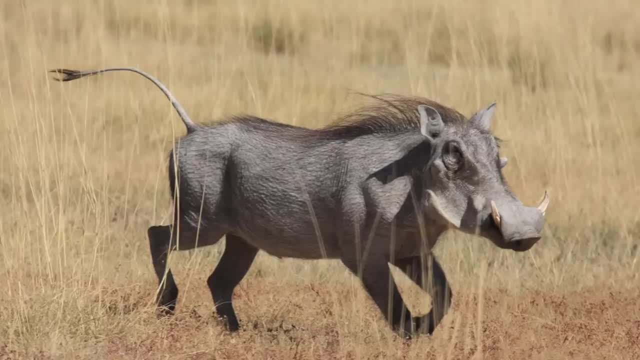 Over 500 different species of birds can be found, as well as mammals like warthogs, aardvarks, hares, gazelles and hyraxes. In terms of predators, Eritrea seems to have more canine species than feline. 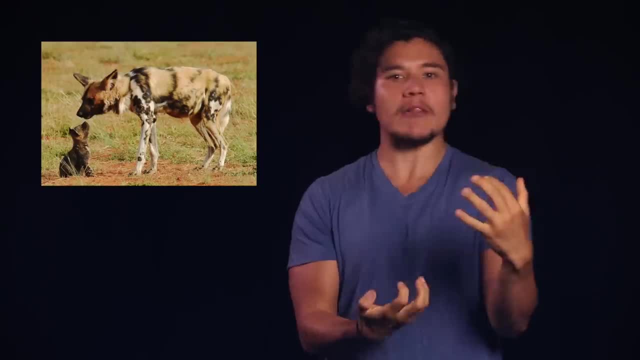 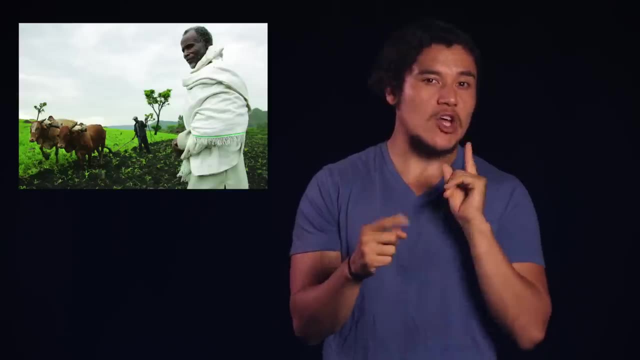 Wild dogs, golden wolves and jackals and hyenas dominate the highlands and plains. Resource-wise, Eritrea actually has a pretty decent, diversified economy. However, two things they thrive off of are livestock and gold, specifically sheeps and goats in the livestock. 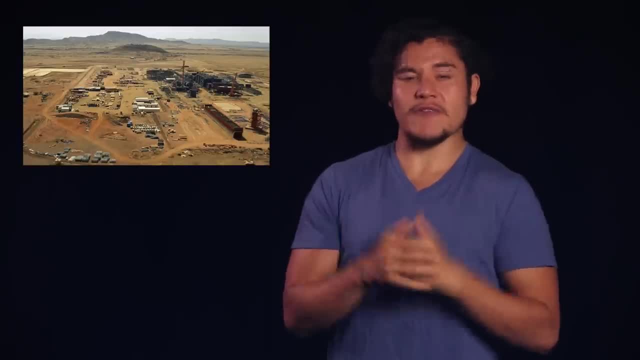 Gold has actually been mined here for centuries and makes up about eh 15 or so percent of the exports. Eh hold on to your horses, though. Even though they have a lot of gold, they still have quite a ways to go in terms of economic development. 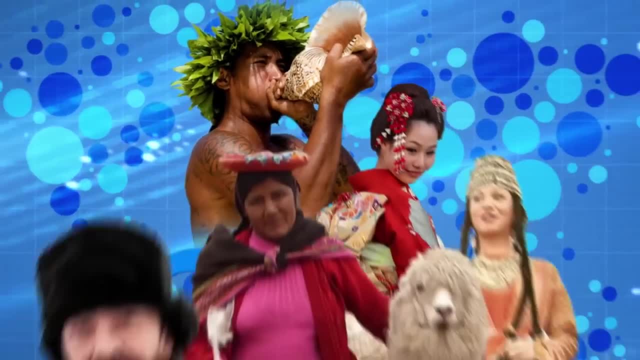 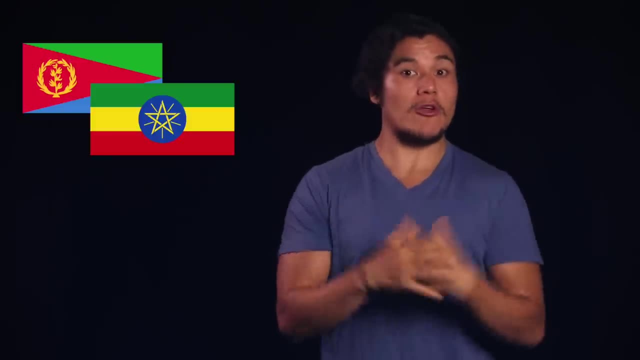 which gets a little controversial. Let's- uh, let's- discuss that in. Okay. so, like mentioned before, Eritreans and Ethiopians will admit that they both have incredibly similar cultures, traditions, belief systems and even language structures. 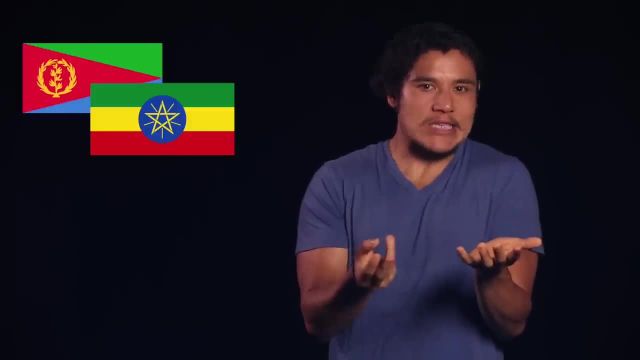 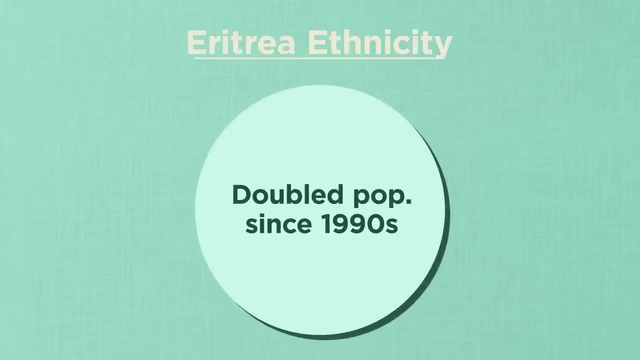 In every reasonable sense they are kind of like cousins. However, do not call Eritreans Ethiopians. First of all. the country has about 6.5 million people and has doubled its population since the 1990s. 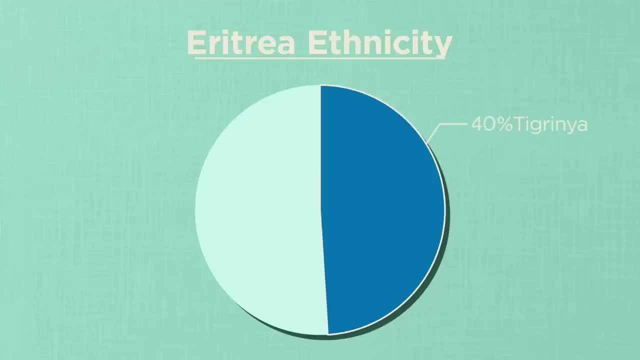 The country is made up of nine distinct ethnic groups, The largest ones being the Tigrinya at 55% and Tigre at 30%, and the remainder come from groups like the Sajo, Kunama, Bilen, Rashida and others. 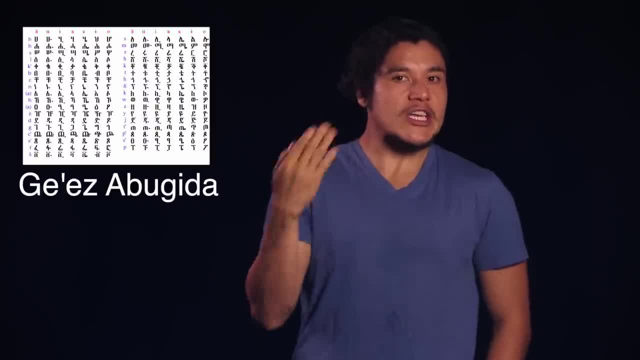 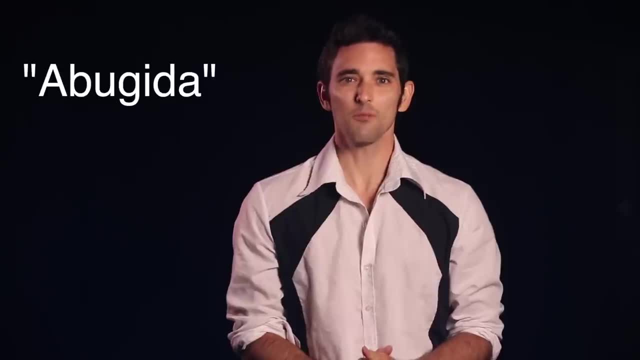 Eritrea is one of the only two countries that uses the only indigenous African writing system in the world that's still used, which, by the way, side note, An abugida is an alphasyllabic writing system similar to Arabic and Hebrew. 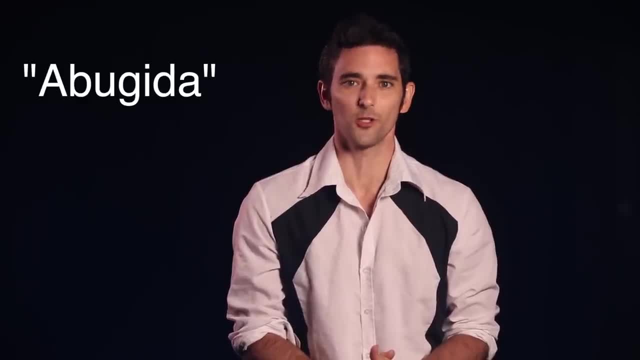 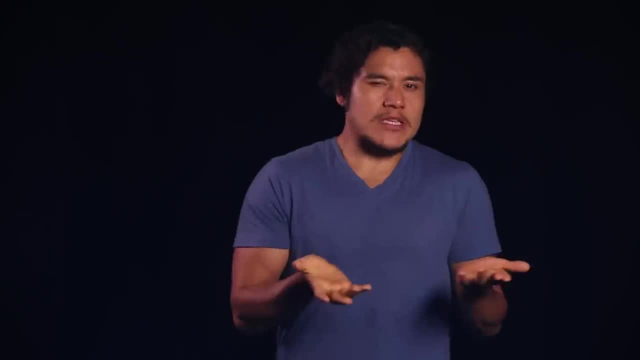 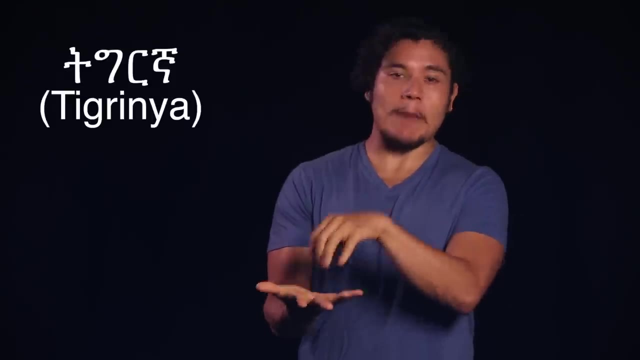 that incorporates consonant-vowel clusters into syllable-character units. The word abugida even came from four letters of the word. So basically, if you want to write something like the word house, it would kind of look something like this: The writing system is used primarily to write Tigrinya, Tigre and Amharic in Ethiopia. 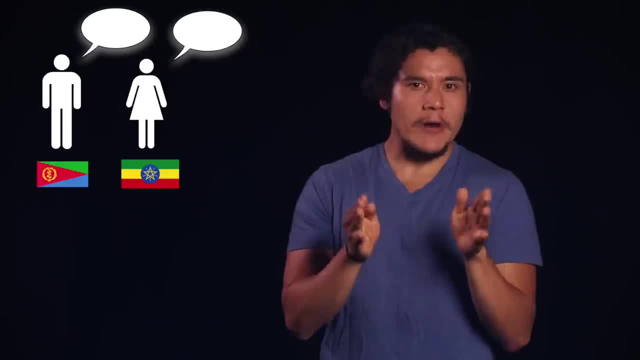 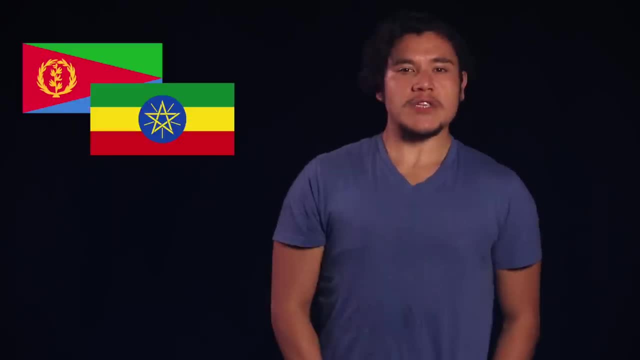 All three languages are pretty similar and if they listen really hard, Eritreans and Ethiopians that speak these languages can kind of understand each other enough to get by. It's kind of like Italian, Spanish and Portuguese. Now here's the thing. 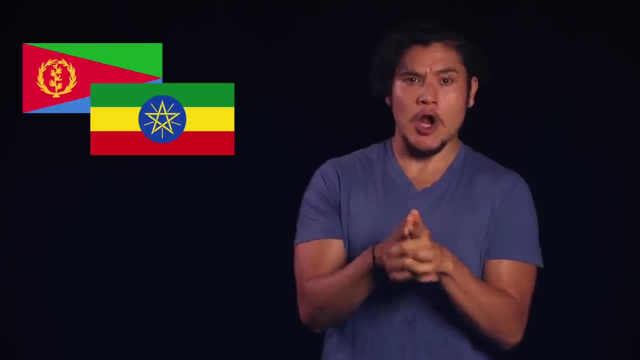 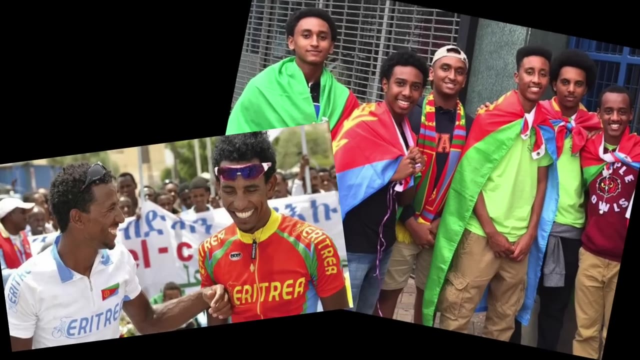 When Eritreans and Ethiopians meet each other, the first question they typically ask is: Are you Habesha? And then they ask which country they're from. So what exactly is Habesha? Habesha people are incredibly unique Semitic, mixed African peoples. 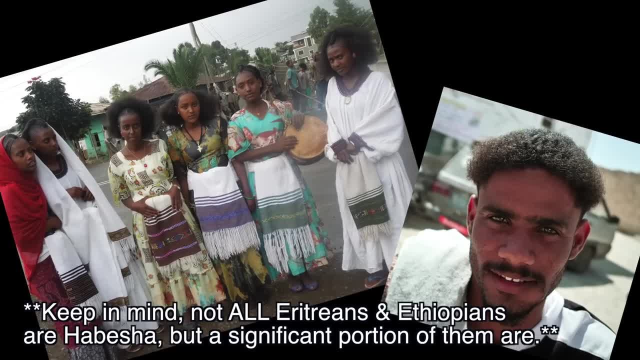 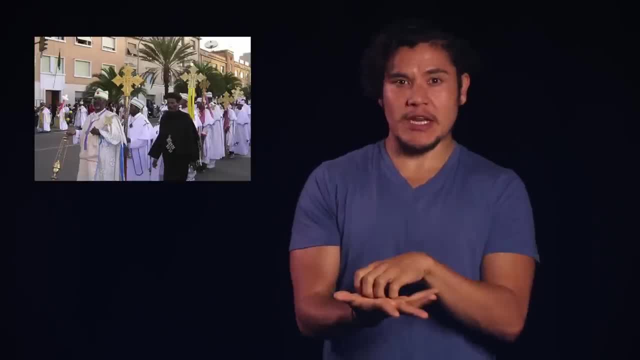 that can only be found in this area. Over millennia, Semitic peoples have mixed in and created this beautiful new group of people found nowhere else: the Habesha. A little bit over half the population adheres to Christianity, predominantly the Coptic. Eritrean Orthodox Church. 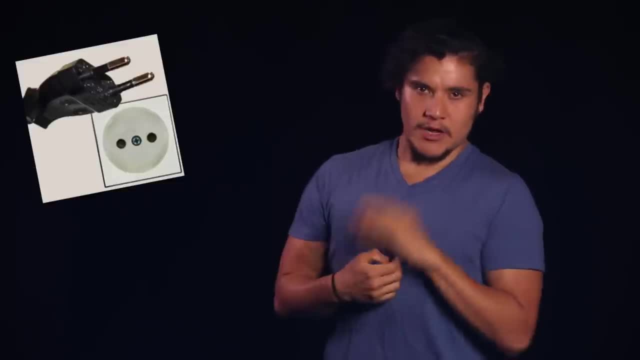 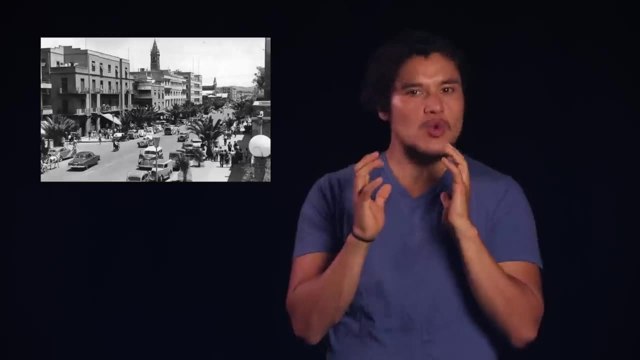 whereas the majority of the remaining population is mostly Sunni Muslim. They also use the Type C plug outlet. they drive on the right side of the road and the currency is the Nafka. Now, because of the Italian occupation, Eritrea kind of has like a little bit of an Italian twang to it. 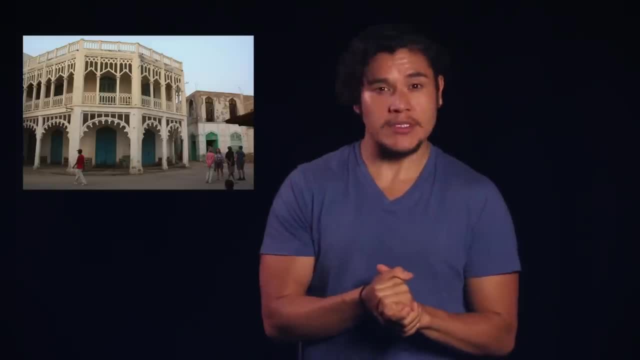 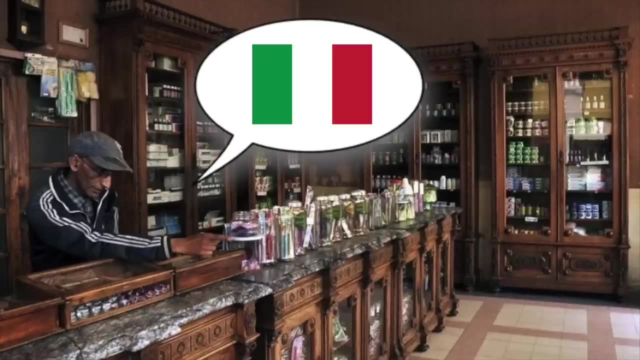 where some of the buildings and shops have clearly influenced architecture. Pizza shops, cafes, and cappuccino and espresso are all over, and many of the residents, especially the older generation in urban areas, can actually still speak and understand Italian. Okay, now, this is where the distinctions are really going to start to come out. 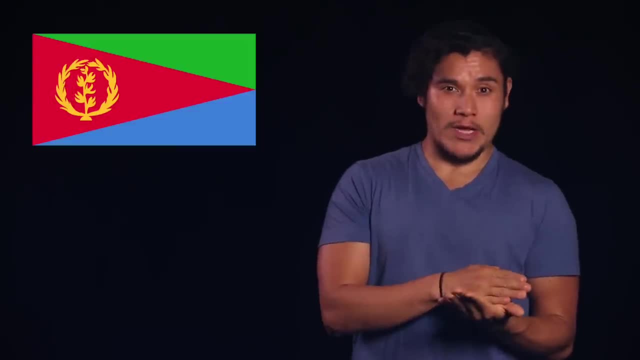 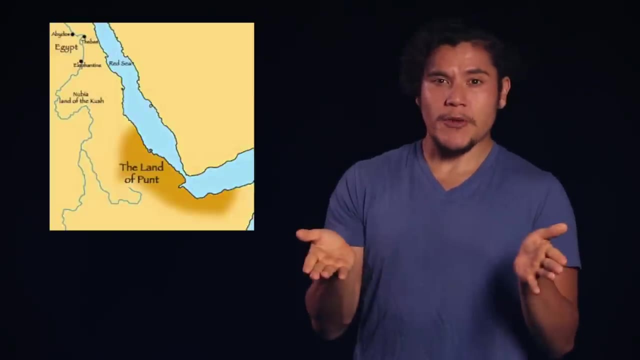 Let's talk politics. Eritrea kind of gets a bad label from the West because of some of the harsh policies that the government adheres to. Some even have gone so far as to label it as the North Korea of Africa, In the simplest way I can put this. the modern day area of Eritrea was most likely the site of the ancient land of Punt. 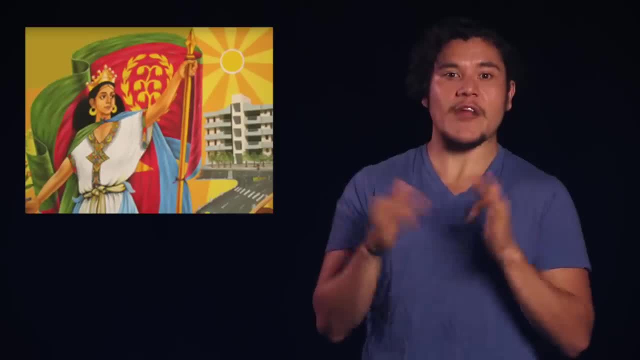 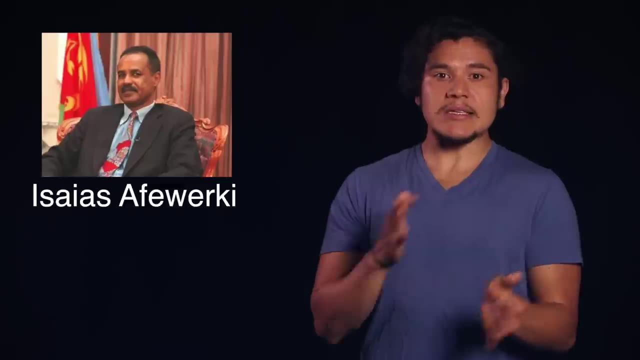 Fast forward after centuries of other empires and nations taking over, until they finally got their independence from Ethiopia in 1993.. Guys, I'm on a time constraint, We don't have time for full historical lessons. Just look it up yourselves: Basically, to this day, Esaias Afwerki has been the president since independence in 1993,. 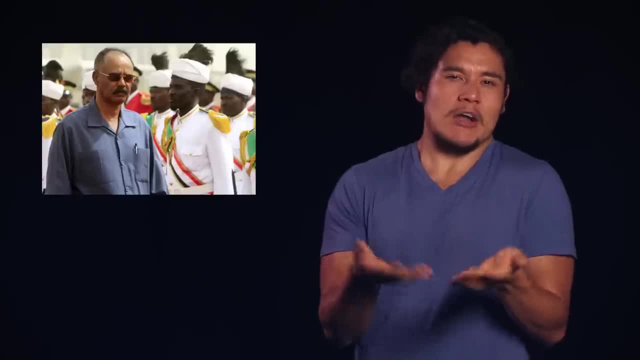 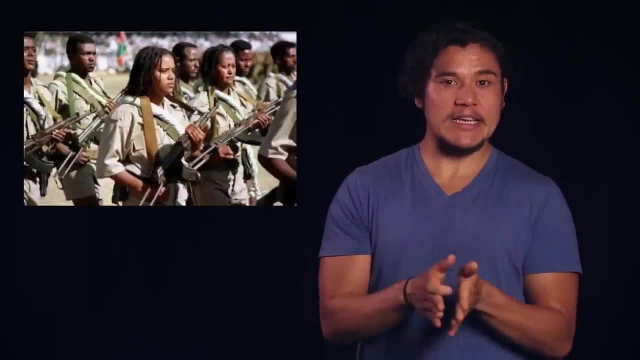 and the country operates in a strange one-party system that has- how can I put this? rather intense social policies. Everybody, male or female, are required to serve military conscription by the age of 18 and continue with national service. It's estimated that about a third of the country's military in the war against Ethiopia were actually women. Originally, national service was supposed to be for 18 months, but the policy changed and now it's kind of like an indefinite amount of time until the government deems complete. This has been a huge hotbed of controversy for many of the citizens, since some have ended up serving for years and really have no say in it. 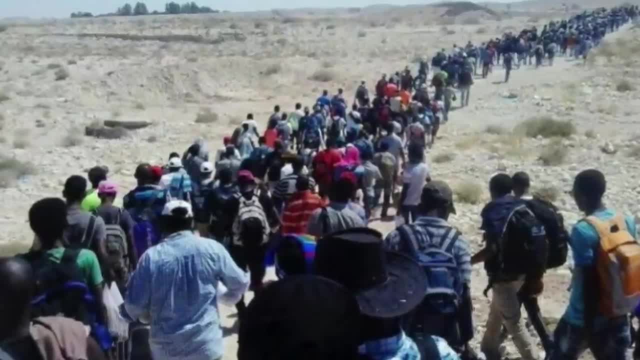 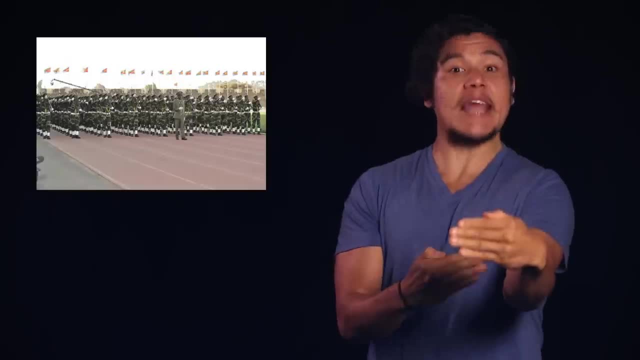 This has also caused quite a few Eritreans to leave on a daily basis to avoid the conscription laws. The government defends itself by saying that they strongly emphasize the strength and wealth of a unified nation that works, moving forward together. This is also one of the reasons why Eritrea doesn't accept most forms of foreign aid. 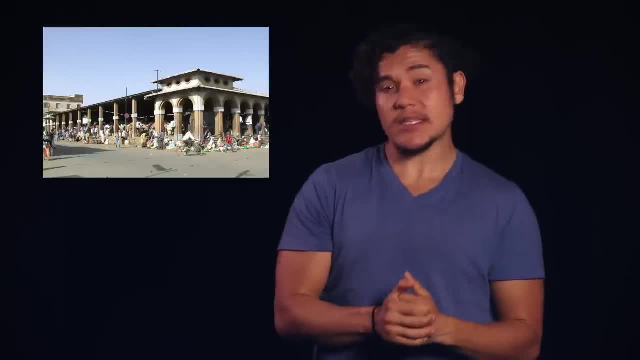 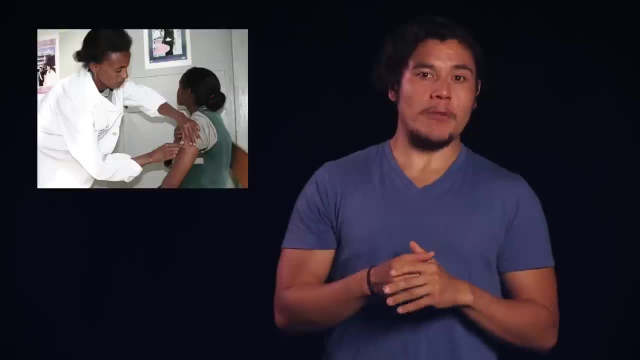 believing that handouts will enable this to happen. The government has actually kind of done a relatively good job at prioritizing the national budget towards education and health, though This has, in return, helped them reach their goals of essentially eradicating polio and most cases of malaria in the entire country.